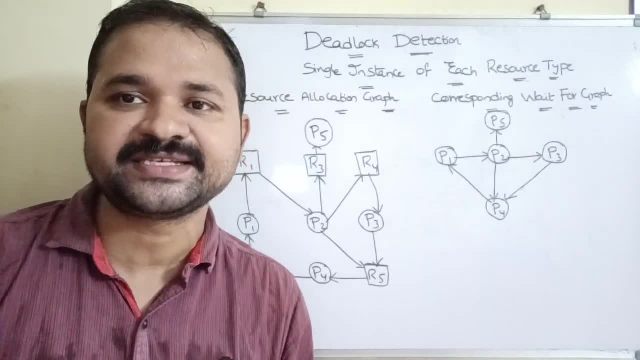 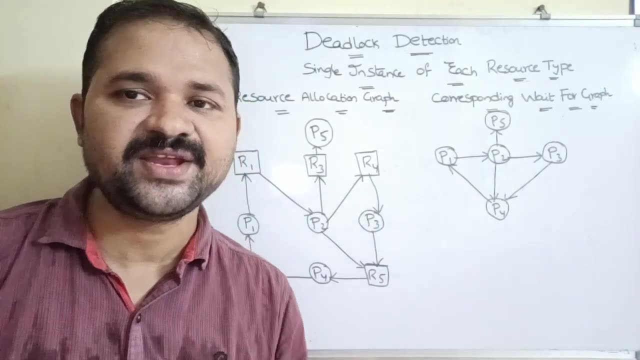 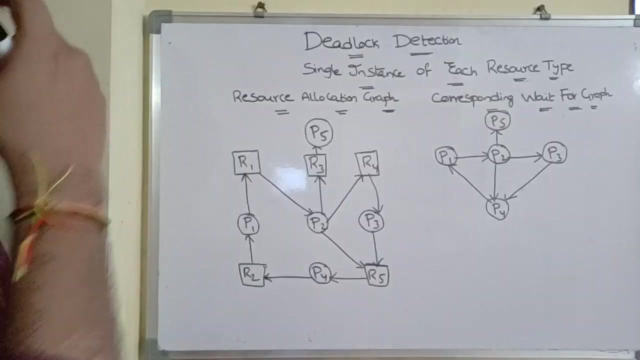 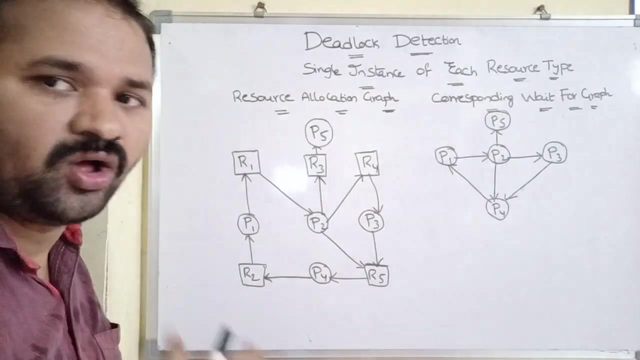 Whereas if the resource type contains multiple instances, then we can use a similar to Banker's algorithm that we will discuss in the next video. So in this video we will discuss about how we can detect a deadlock if the resource type contains a single instance. So let's see this one. So deadlock detection if single instance of each resource type, So if all the resource types in the graph contains a single instance. So this is resource allocation graph. 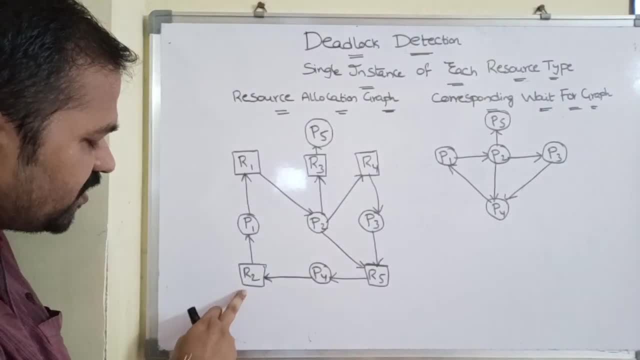 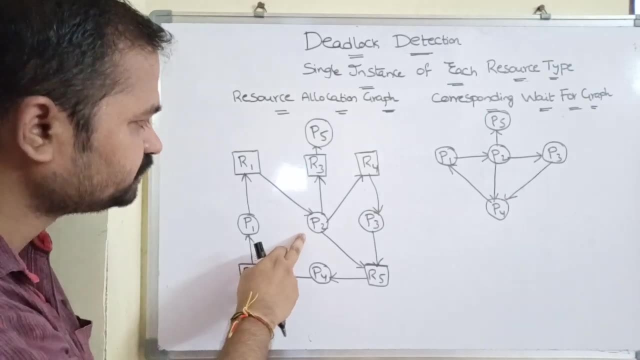 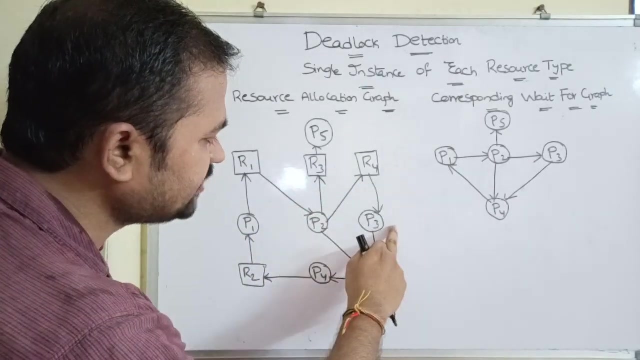 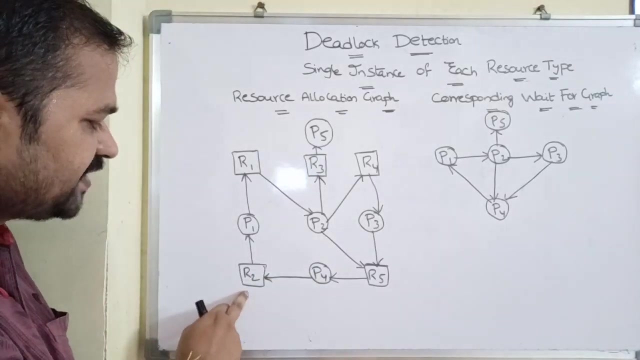 So this graph specifies that P4 is waiting for R2, but R2 is allocated to P1.. Next to P1 is waiting for R1, but R1 is allocated to P2.. P2 is waiting for R3.. R3 is allocated to P5.. P2 is waiting for R4.. R4 is allocated to P3.. Next to P3 is waiting for R5.. R5 is allocated to P4.. Next to P4 is waiting for R2.. R2 is allocated to P1.. So this is our resource allocation graph. 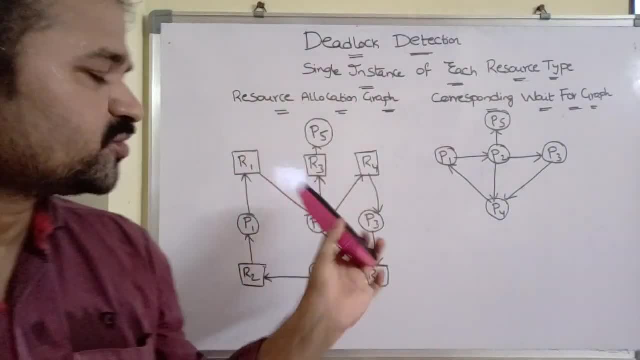 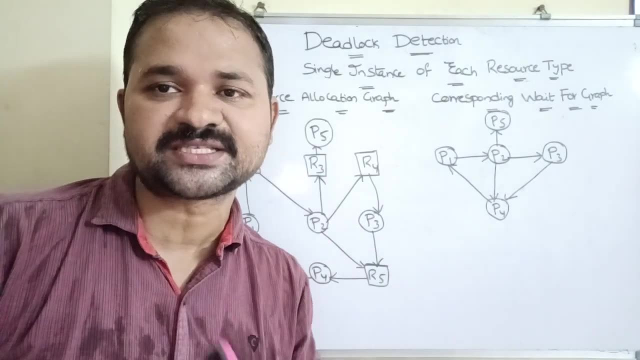 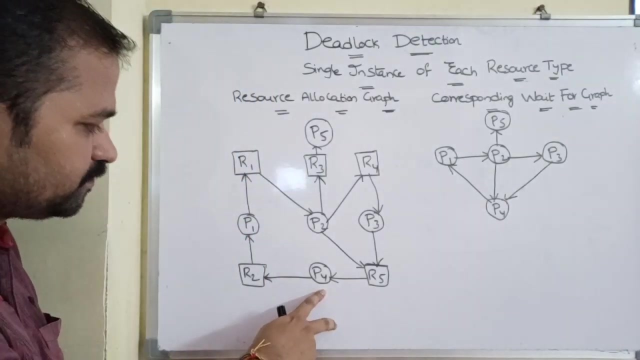 to construct wait for graph for the corresponding resource allocation graph. here, construction of wait for graph is very, very simple. simply, we have to remove the resources and connect the processes. if we observe about p1, so let's observe about p4. so p4 is waiting for r2, but r2 is allocated to p1, so we 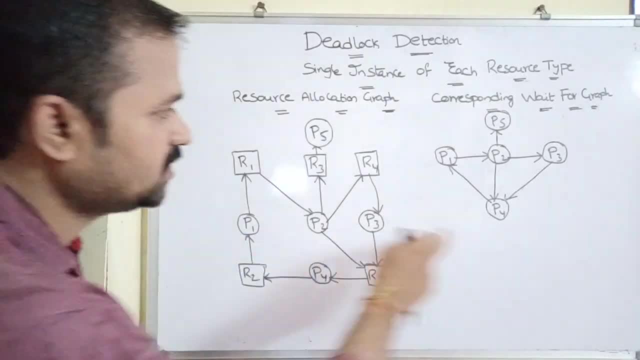 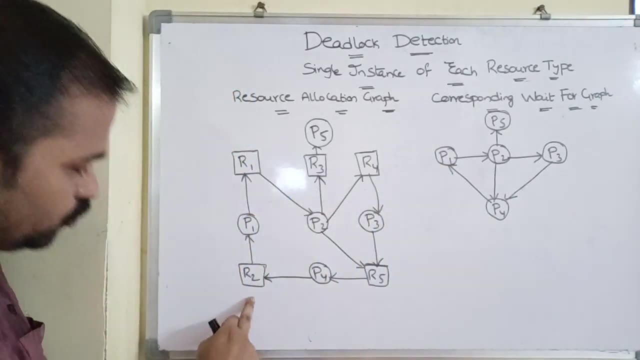 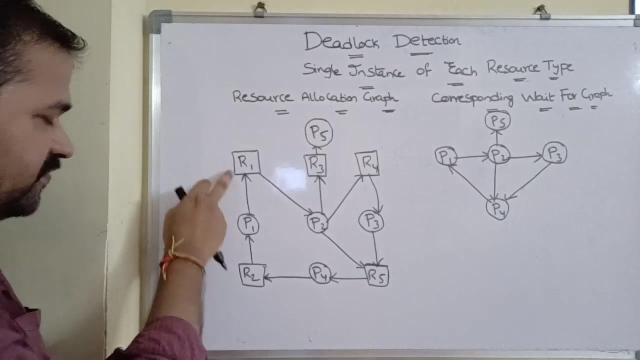 have to remove this r2 and connect these two. so p4 is waiting for. so p4 is waiting for a process, p1 to release the resource r2. likewise, if you observe about p1, p1 is waiting for r1, but r1 is allocated to p2, so we can remove this. 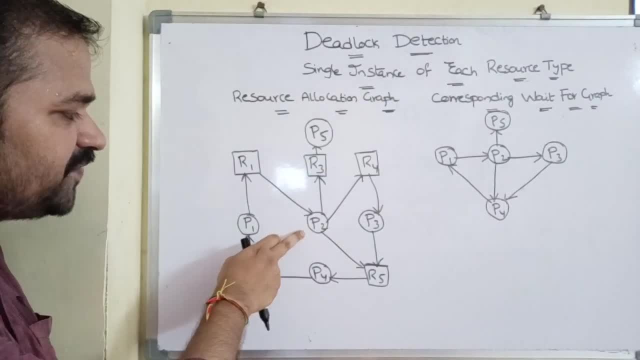 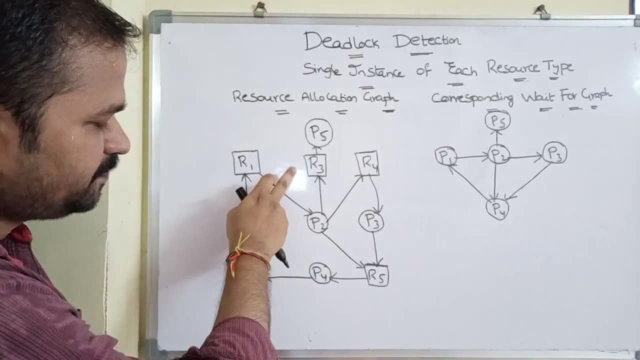 resource and we can write as: p1 is waiting for p2 to release r1, so p1 is waiting for p2. next, if you observe about p2, p2 is waiting for r3, but r3 is allocated to p5, so we can remove this r3. so we can write as p2 is waiting for. 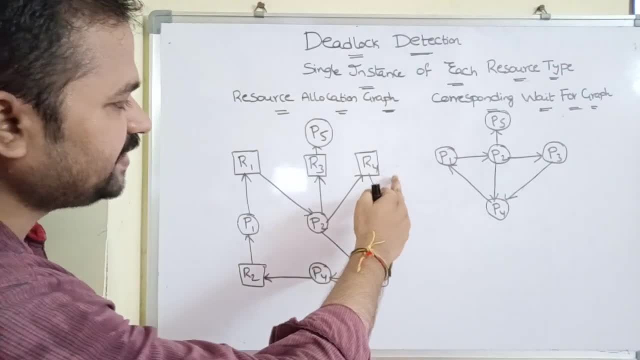 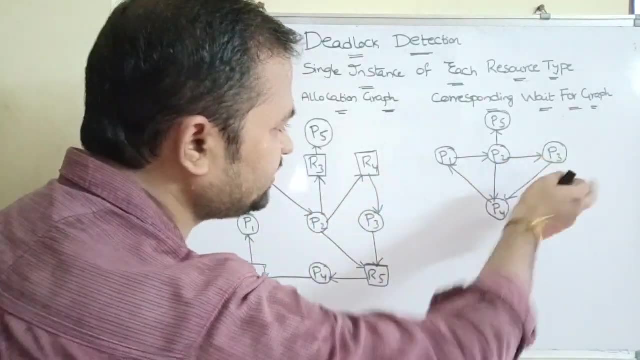 p5. so likewise, p2 is waiting for one more resource, r4, but r4 is allocated to p3, so we can remove this one and we can write as p2 is waiting for p3. so likewise we have constructed wait for graph. after constructing, wait for graph operating.